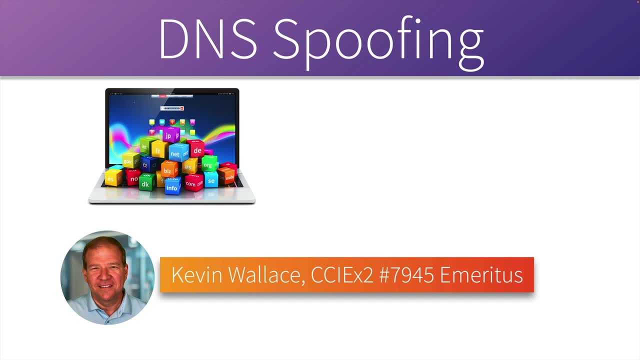 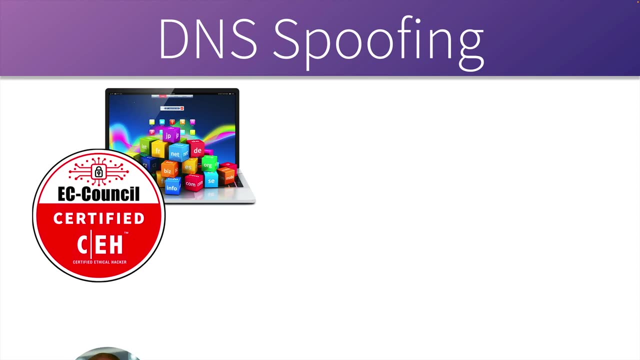 which is called DNS Surveillance. We'll see how an attacker might launch such an attack and we'll talk about how we can defend against this attack And DNS spoofing. that's a topic appearing on the CEH, the Certified Ethical Hacker Exam Blueprint. So if you're preparing for that exam- to be a certified ethical hacker- 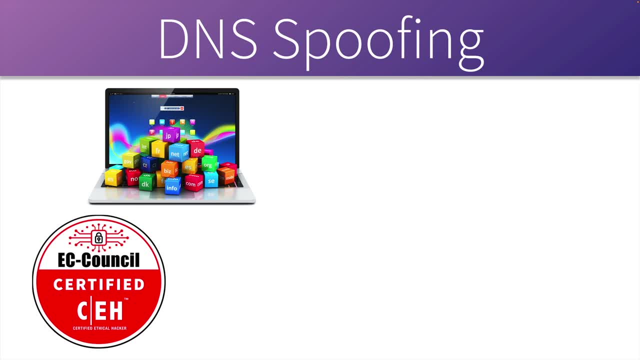 you'll want to know how DNS spoofing works, Or if you're just concerned about better protecting your enterprise environment from DNS spoofing, this is the video for you, And we're going to begin by taking a look at an overview of DNS spoofing. We will walk through a hypothetical example and then we'll see how an attacker might. 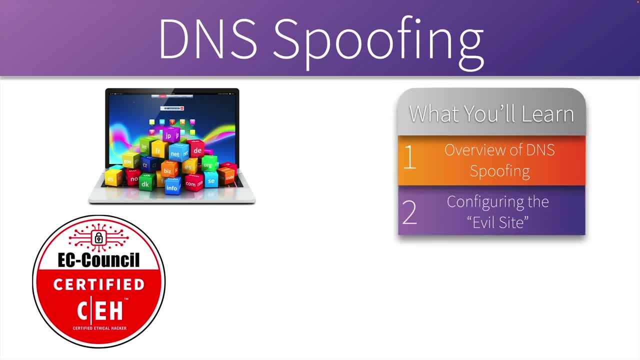 set it up. We'll go in to Kali Linux and, using Apache, we're going to set up a fake website- that is going to say evil site when we land on it, And we're going to configure a utility that an attacker might use, called Ettercap, And we'll see how they might use that to perform a DNS spoofing. 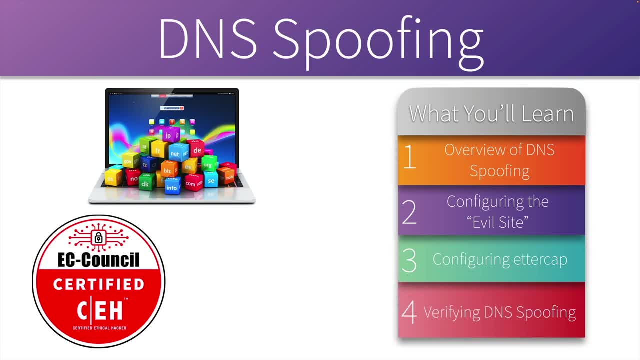 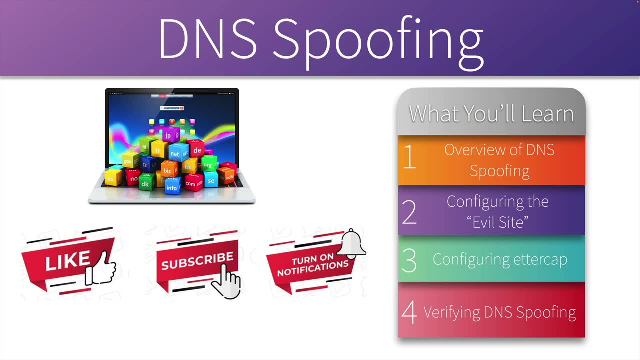 attack And then we're going to verify that the DNS spoofing attack was successful. And if you enjoy this video and find it valuable, please subscribe to our channel and turn on notifications so you don't miss any of our future content And since we are dealing with a utility that could be used for bad purposes. 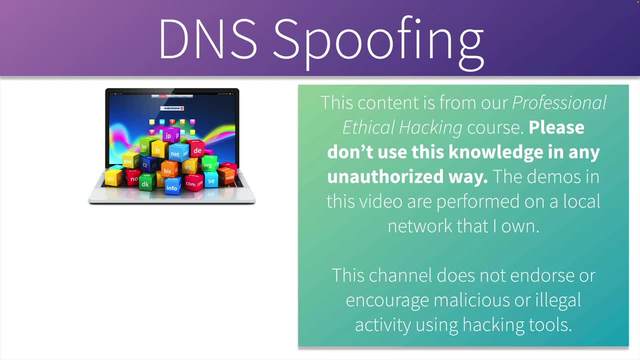 I want to make my intent very clear. The content that you're about to see is from our professional ethical hacking course, And I encourage you to not use this knowledge in any unauthorized way. I am performing the following demonstration on my local equipment that I personally own And this channel definitely does not endorse. 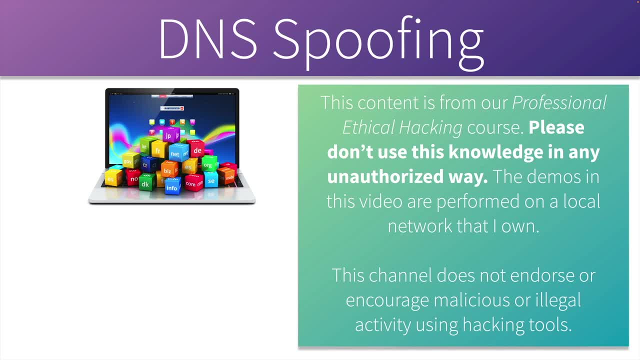 or encourage malicious or illegal activity using hacking tools. In fact, it's just the opposite. I want to show you how to protect yourself against these types of attacks, And this DNS spoofing attack can be defeated using a couple of utilities we talked about in a prior video here on the 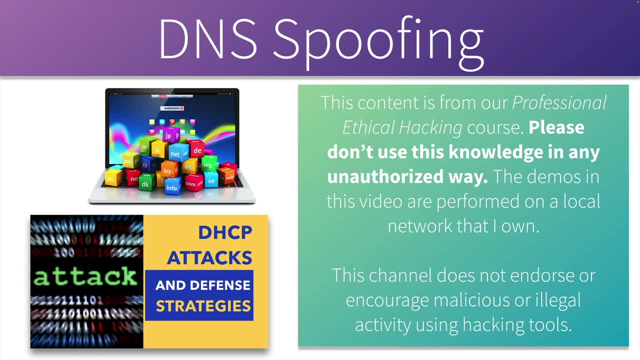 channel called DHCP Attacks and Defense Strategies And I'll leave a link to that video in the description. So after you watch this video you may want to go through that other video where I set up the defense strategies. In that video we show you how to set up a couple of features. 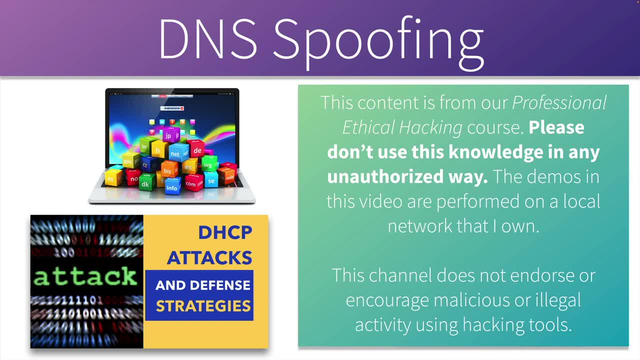 called port security and DHCP snooping, And those are the features we could use to prevent a DNS spoofing attack, as we'll talk about in this video. And I'm not sure when you're watching this video, but if you happen to be watching it before September 28th 2022, then I would like 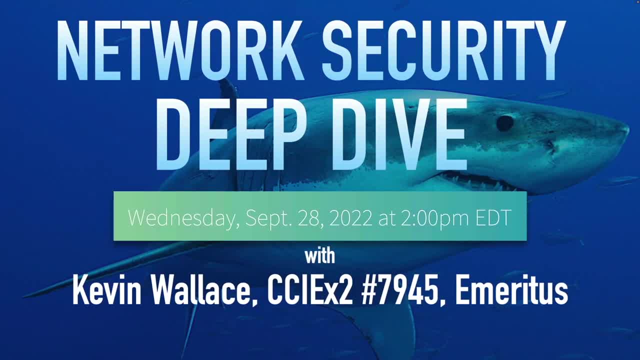 to invite you to a completely free deep dive training session that we're doing. It's going to be on Wednesday, September 28th 2022.. It's going to be at 2 pm Eastern Daylight Time, And Eastern Daylight Time is UTC minus four. 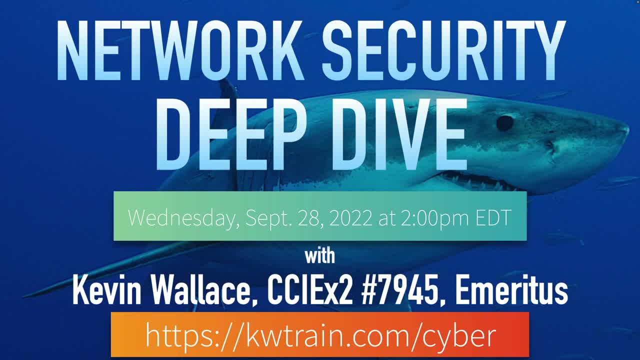 So this completely free deep dive event, which I believe is going to be our longest deep dive ever, we're going to cover a ton of security topics. Just go to kwtraincom slash cyber Again. that's kwtraincom slash cyber. Now let's get into this week's video on DNS spoofing. 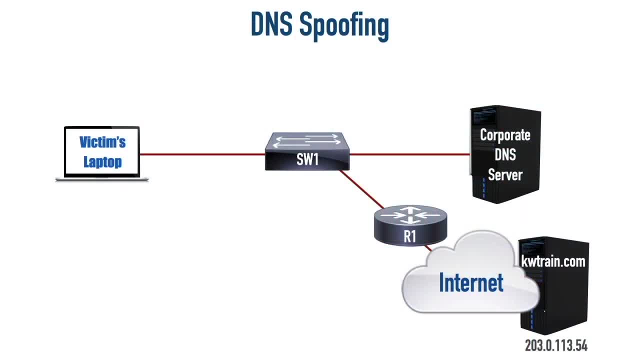 In this video let's consider an attack called a DNS spoofing attack. This is known by another name. It's also known as a DNS cache poisoning attack. To begin, how DNS functions. We've got this laptop on screen and let's say it wants to go to kwtraincom. 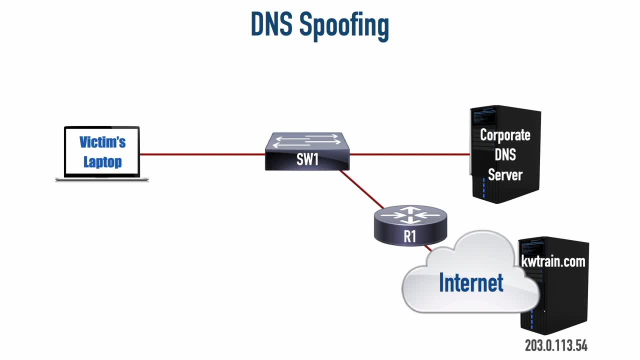 out on the internet but it doesn't know the IP address of the kwtraincom web server. So that laptop is going to go ask its DNS server. hey, can you tell me the IP address corresponding to the name of kwtraincom? The DNS server receives that and it responds. 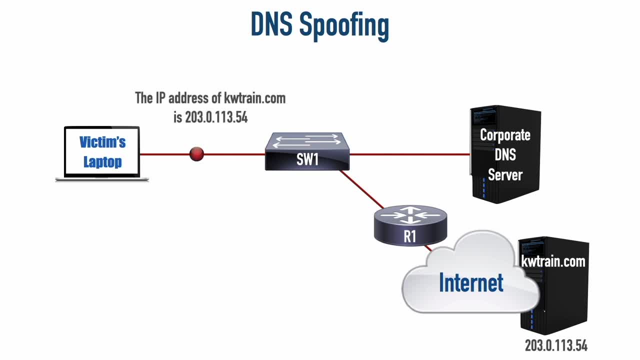 with a message saying: yeah, that's at 203.0.113.54.. That goes back to the laptop and the laptop is going to cache the IP address, So that's going to go ask its DNS server. hey, can you tell me the IP address corresponding to the name of kwtraincom? 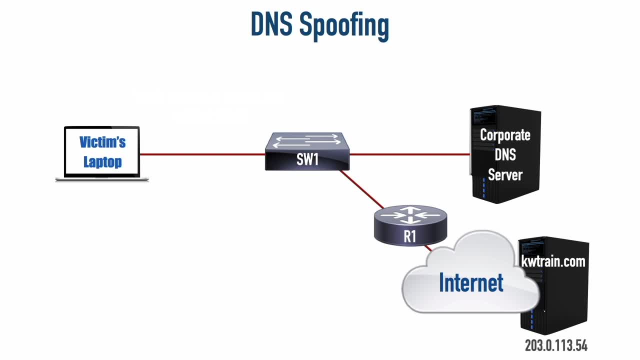 For a period of time locally, And now, when it wants to go to kwtraincom, it knows the corresponding IP address that can be routed out to the internet. However, let's say an attacker wants to put up a lookalike page. They have a web server and they want to make it look like kwtraincom. 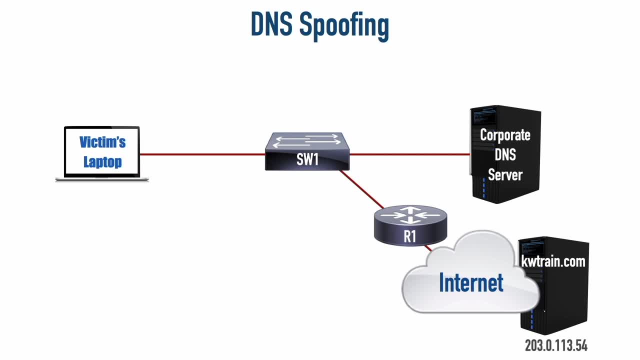 So when somebody goes to log into kwtraincom they'll actually be logging in to the attacker's website. Let's say the attacker attaches a web server with an IP address of 172.16.. dot 101.150.. But the question is, how can that attacker cause the victim's laptop? 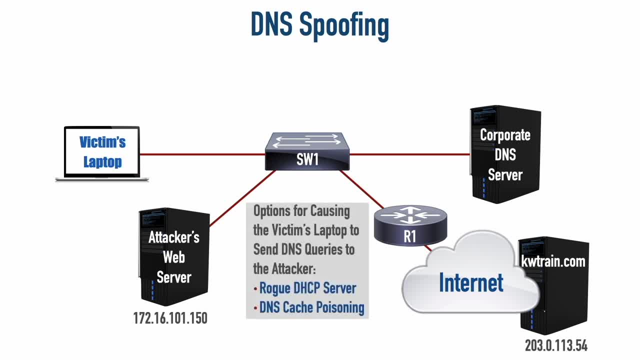 to go to the attacker's web server. Well, one option is they might connect a rogue DHCP server to the network, As we previously discussed. if the victim's laptop learns IP address information from that rogue DHCP server, it might learn the IP address of a DNS server, which is actually 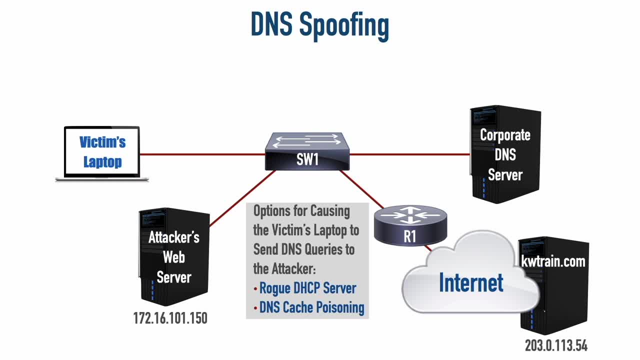 a DNS server set up by the attacker which is going to direct the victim to the attacker's web server When the victim is attempting to go to kwtraincom. And another option that I don't have listed here is if the attacker gains access to the victim's laptop, they could update the local hosts file. 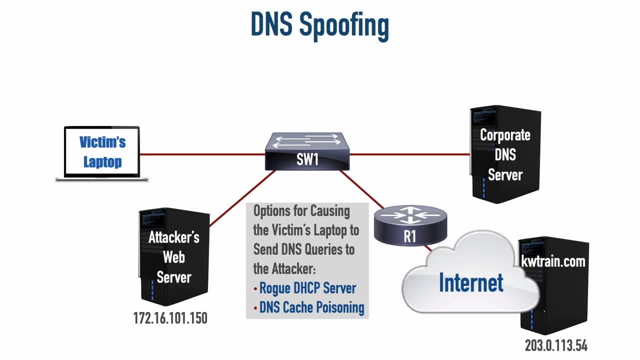 on that laptop. That's going to take precedence over any DNS lookup. But, assuming the attacker does not have access to the victim's laptop, something else they could do- and that's what we're going to demonstrate in this video- is DNS cache poisoning With DNS cache poisoning. 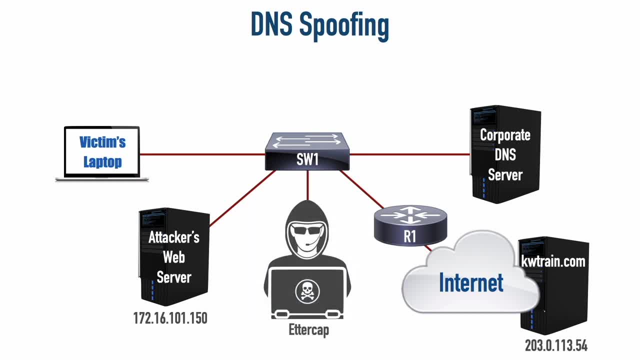 the attacker might be running utility such as EtherCAP- or EtherCAP, depending on how you want to pronounce that- And if they first launch a man-in-the-middle attack, as we previously demonstrated with EtherCAP, traffic flowing between the victim's laptop and the DNS server is going to flow. 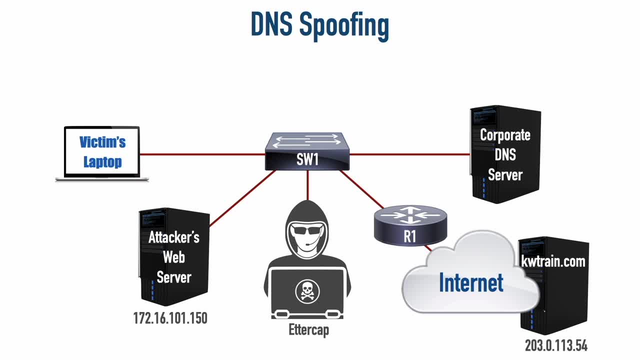 through the attacker if the attacker specifies the victim's laptop as one target and the DNS server as another target. So now, when the victim's laptop tries to resolve the IP address for kwtraincom, it's going to go to the attacker, who's going to respond with a message. 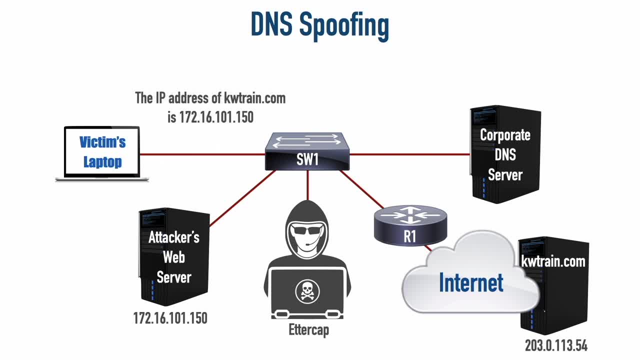 saying: Oh yeah, kwtraincom that's at 172.16.101.150.. Their fake web server that is set up as a lookalike web server to kwtraincom, attempting to capture the login credentials of the victim. 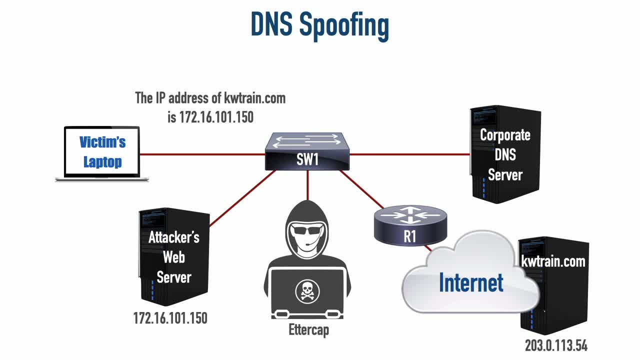 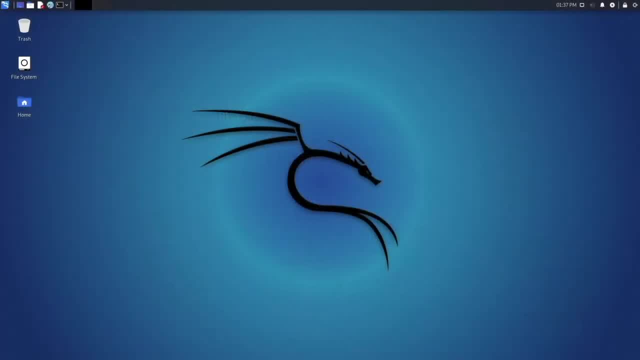 Now let's go out to a live topology and see how an attacker might pull off a DNS spoofing or, as it's also known, a DNS cache poisoning attack. And here we are sitting on our Kali Linux box. This is going to be the attacker's machine. we're 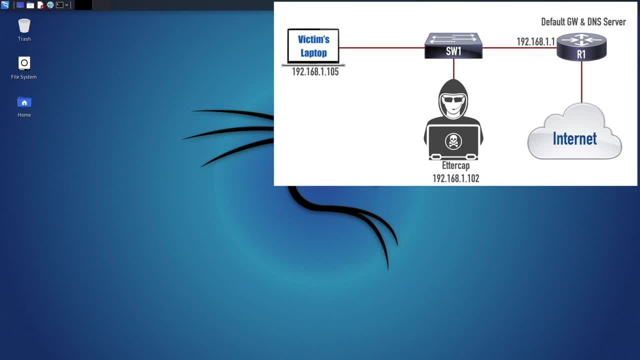 pretending And we're going to set up, just as a basic example, a fake kwtraincom website on this machine, Just to demonstrate that we could redirect DNS queries looking for kwtraincom. we could divert those to another site. So we're not going to go through the process of setting up a lookalike site. I'm 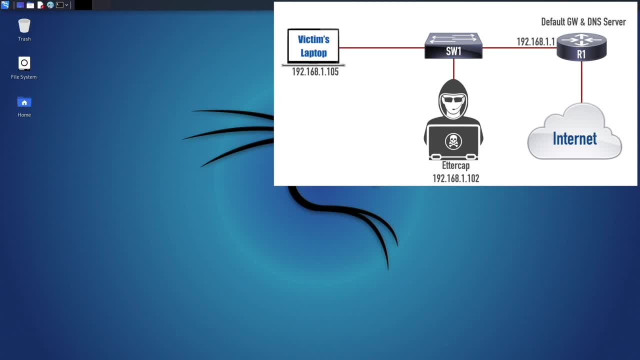 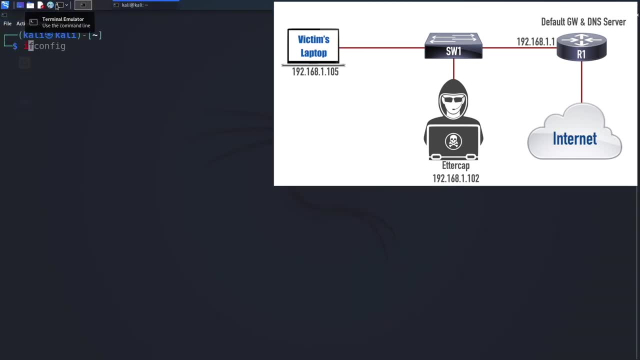 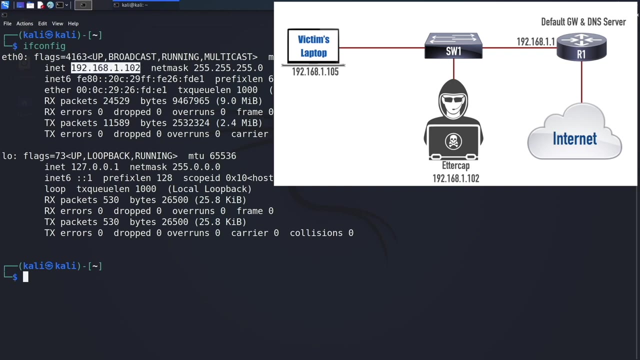 just going to set up a basic page so we know that, yep, our traffic has been diverted. First let's see what the IP address is on this Kali box. Let's go open up a terminal and I'll say ifconfig, And it looks like our IP address is 192.168.1.102.. 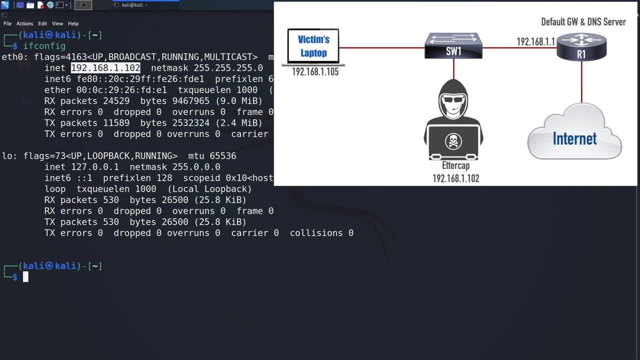 Now let's start the Apache web server on this machine. To do that, I'll do a sudo service, apache2 start, And I'll give my superuser password. And just to demonstrate that this page is up and functioning, let's go over to the victim's laptop. 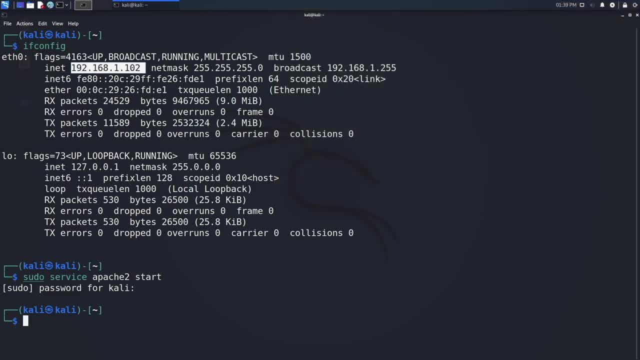 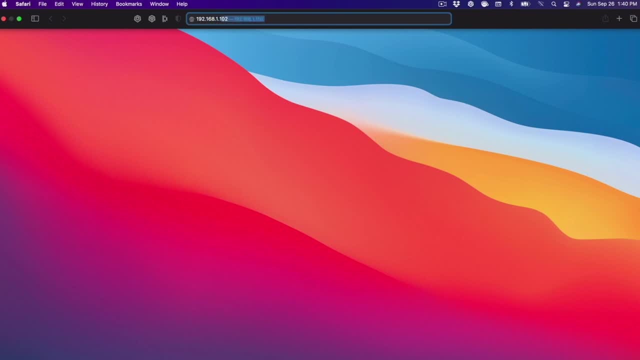 And directly point to 192.168.1.102.. Here on the victim's laptop, let's go to 192.168.1.102.. We'll press enter And that is the default web page for our Apache 2 server. 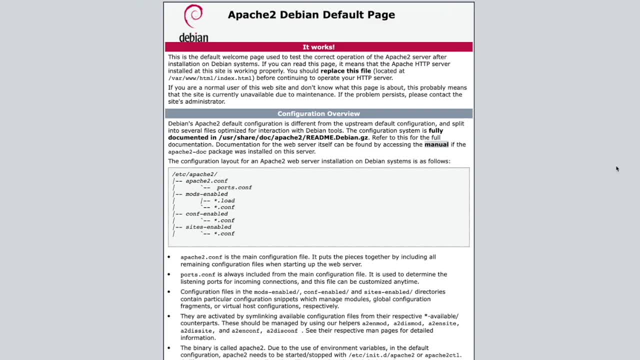 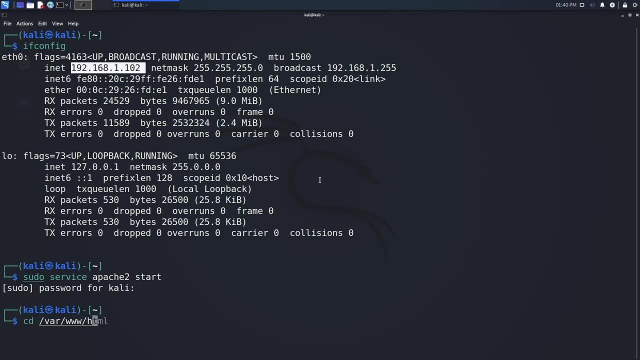 Now let's go back to our Kali box and really quickly change that page to something that we create. So back on our Kali box. I'm going to cd into slash, var, slash, www, slash, html. Let's list the files in this directory. 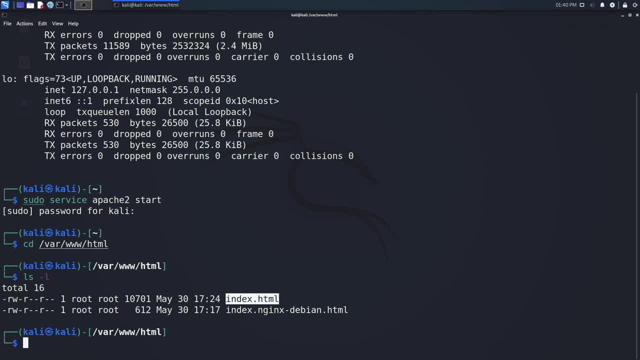 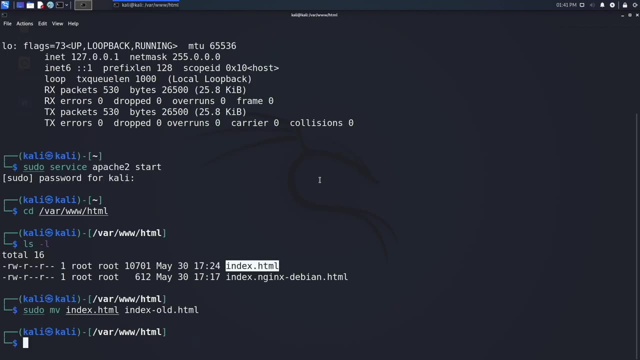 I'm going to edit this indexhtml file. In fact, let's move this to a backup file and I'll create a brand new indexhtml file. Let's do a sudo, move indexhtml to index-oldhtml. And now let's create our own indexhtml. I'll do a sudo and I'll use the vi editor. You can. 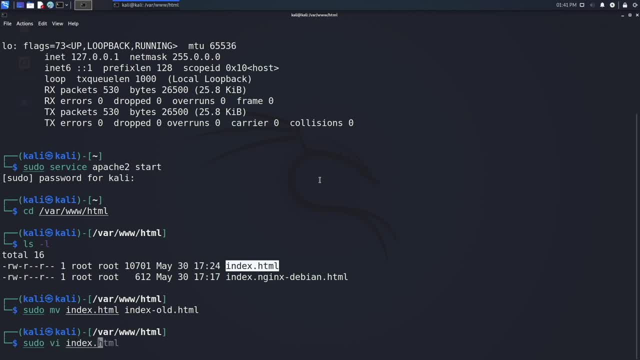 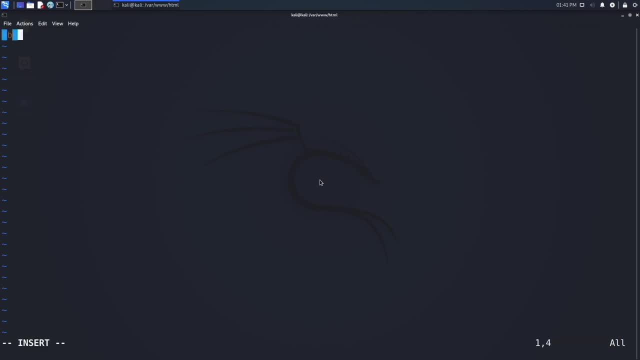 use whatever editor you like on Kali Linux. I'll say indexhtml And I'm going to make this super I to insert, And then I'll give a bold tag And I'll say evil site. Then I'll do a slash b to 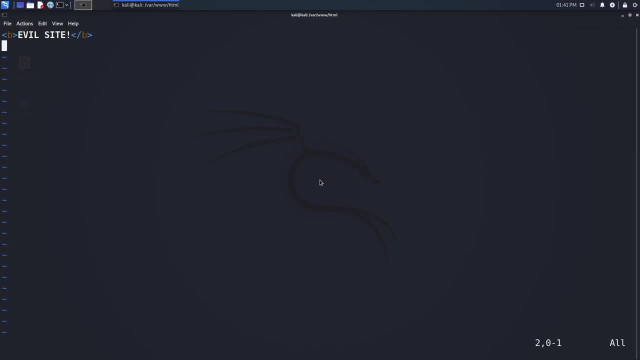 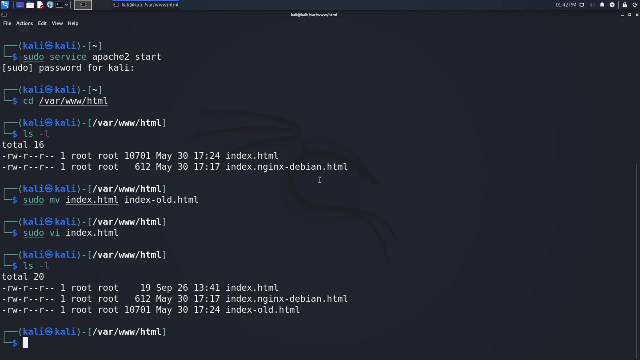 close out the bold tag And that's it. I'll do an escape colon: wq to write and quit. Let's make sure that file does exist. It's readable by everyone. Awesome. And to confirm, this web page is showing up on our victim's laptop. let's go back over to the victim's laptop And let's reload. 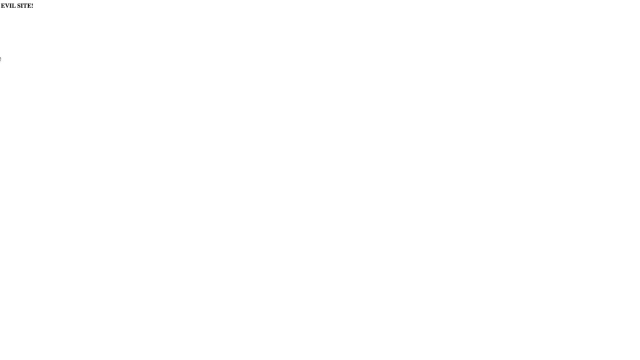 192.168.1.102.. And it comes back and it says evil site. And now that we have our evil site set up, let's discuss how we can use Ettercap to resolve DNS queries coming from our victim's laptop wanting to get the IP address of kwtraincom. Then Ettercap is going to respond to the DNS query. 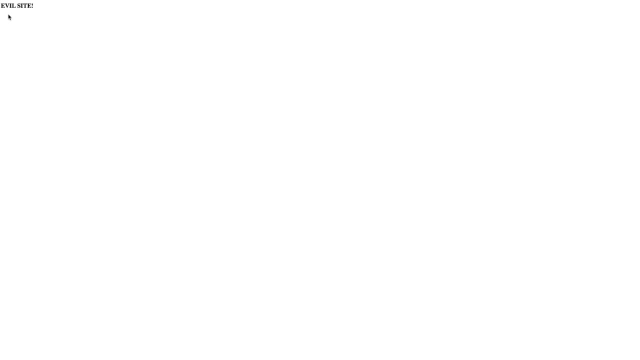 with a reply saying that its address is 192.168.1.102, the address of our Kali box. Now, before launching Ettercap, we've got some work to do on a couple of the Ettercap configuration files. 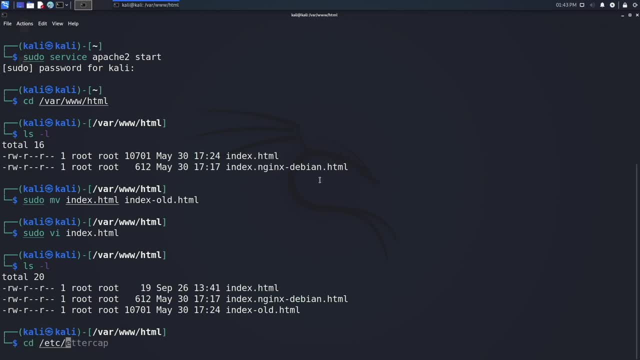 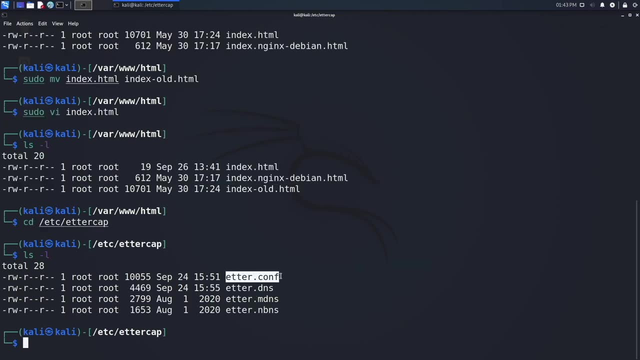 So let's go back to our Kali box and let's go into the etsy slash Ettercap directory And we need to edit both the Etterconfiguration, or cunf file and the Etterdns file. First let's edit this configuration file. We'll do a sudo vi Ettercunf And the first thing I want: 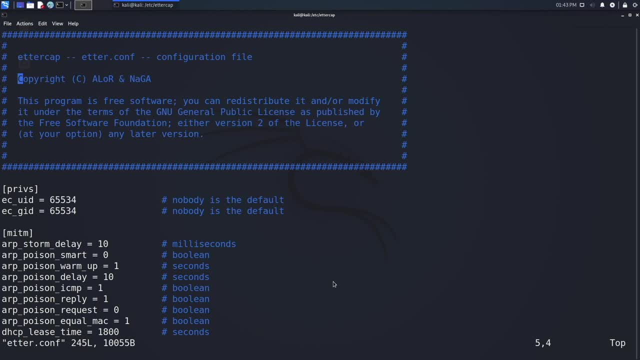 to do is to give Ettercap permissions to do all the things that we want it to do, And to do that, I need to change this user ID and this Group ID. I'm going to change those to zeros, So I'll delete those values. insert a zero. delete those values. insert a zero. 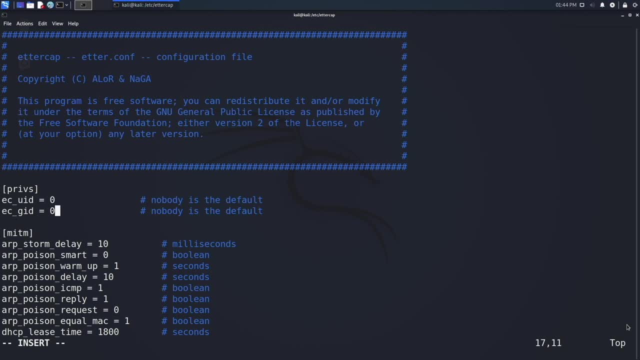 And next, there are a few lines that I need to uncomment, meaning I need to get rid of the pound sign in front of them. that makes them a comment. You see, the lines I want to uncomment are specific to the operating system that we're running on. 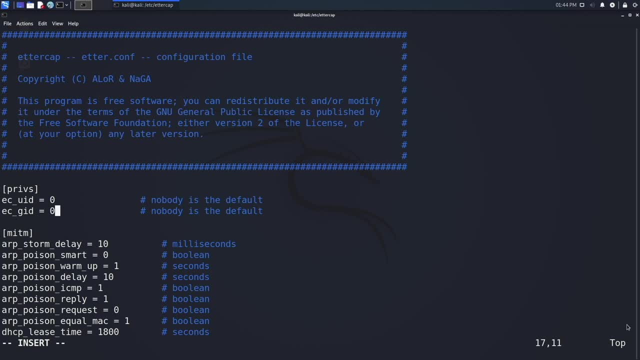 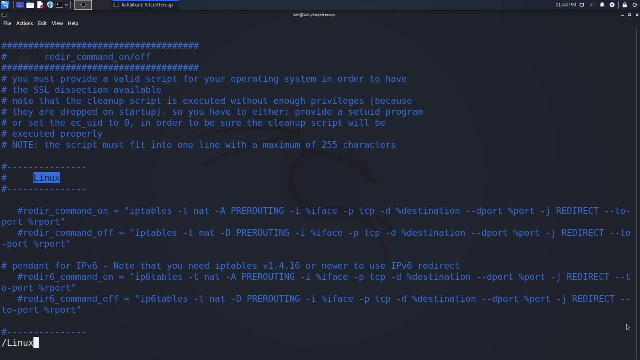 Now I'm running on Kali Linux, so I want to uncomment the lines for Linux. To jump down to that configuration section. I'll do an escape forward, slash Linux And I've got these four lines. I want to remove the pound sign from. 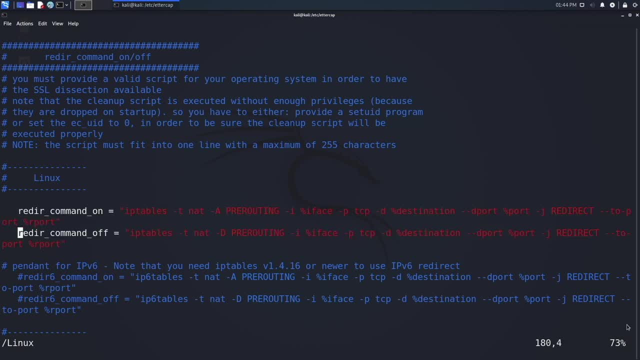 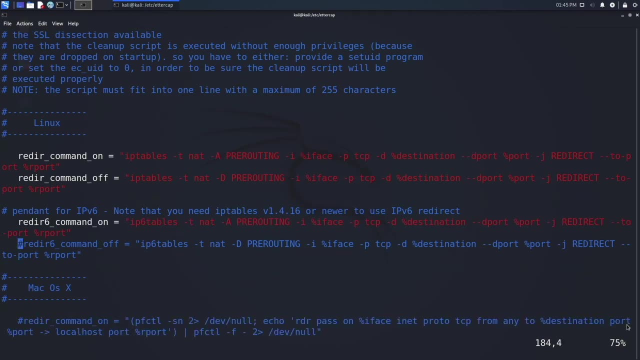 So I'll get rid of that pound sign and this one Common mistake here. you also need to get rid of the pound signs in front of the IP version six lines that are commented out. So I got rid of those four different pound signs. 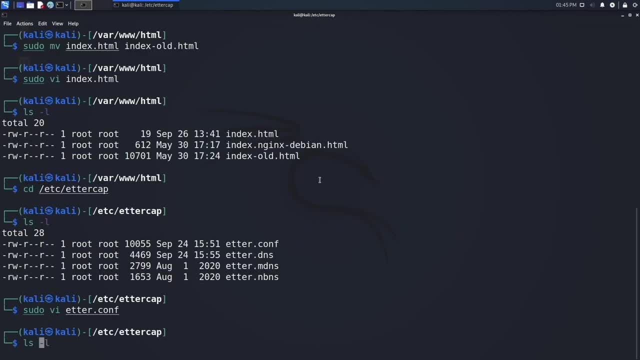 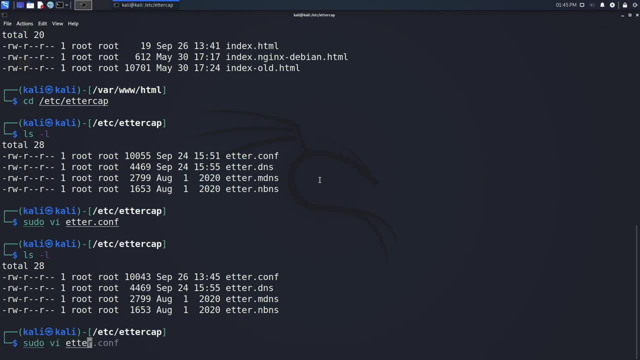 Let's do an escape colon WQ, And now I need to edit that editordns file. So I'll do a sudo vi editordns And I'm going to go down to the very bottom of this. You can read through this if you'd like more information. 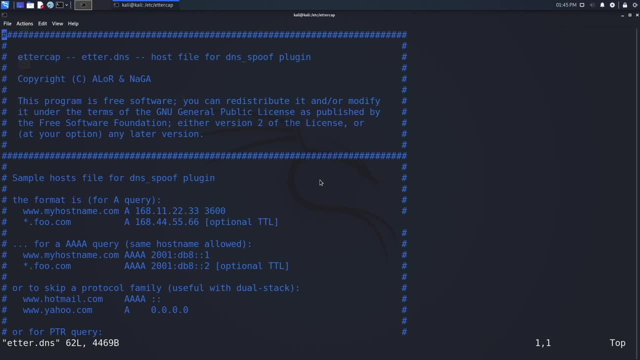 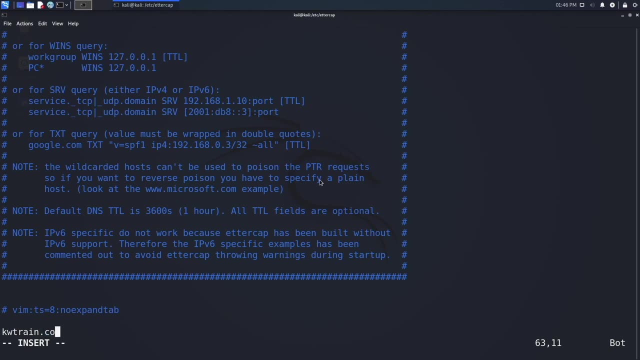 on how to do the formatting. But to get to the very bottom, I'll do an escape, then a shift G, I'll do an O to add a new line And I'll say kwtraincom, and I'll make this an A record. 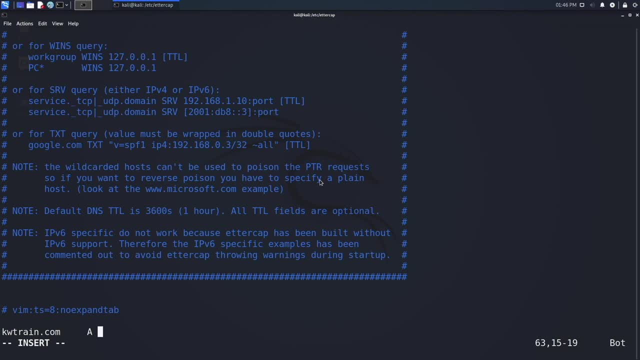 So I'll do a tab, capital A, And I'll say: if you want to go to kwtraincom, go to 192.168.1.102, which is the address of this Kali box. Next I'll say starkwtraincom. 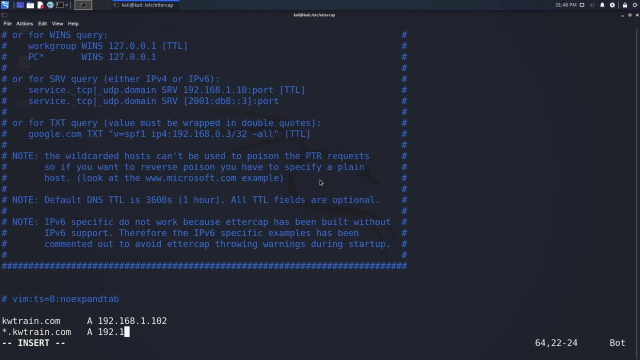 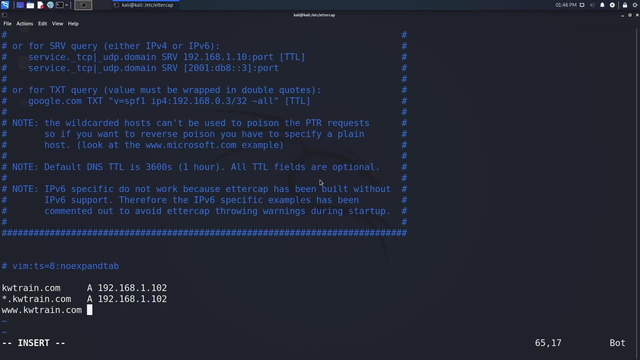 This is also an A record And we'll say: go to 192.168.1.102.. And let's do one other line. I'll do wwwkwtraincom. This time it's a pointer record, PTR. 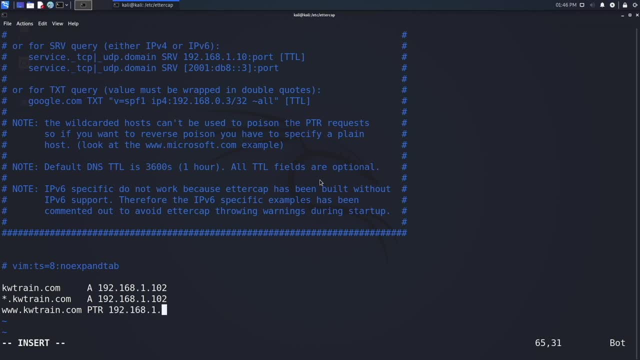 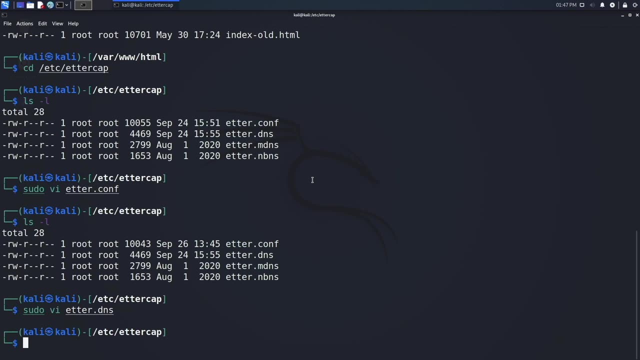 And it's going to go to 192.168.1.102.. Escape colon, write quit And we're done. And before running Ettercap, let's make sure that our laptop is getting to the actual webpage that we want. 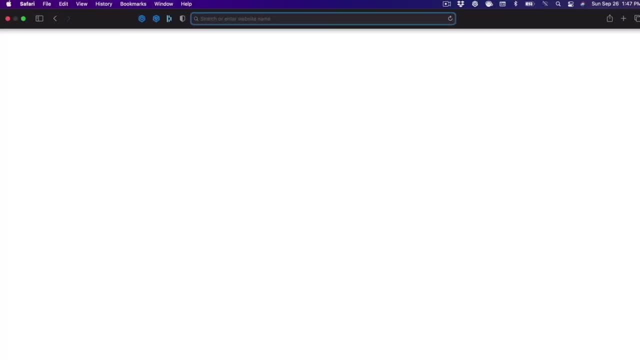 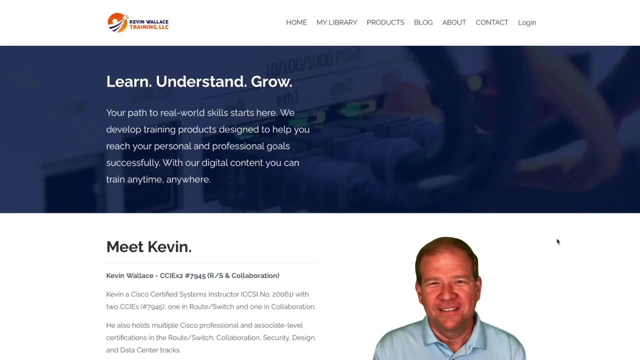 So let's go back to our victim's laptop again, And I'm going to go to wwwkwtraincom And there's my webpage, perfect. And in this example, as is often the case, the victim's laptop is using its default gateway. 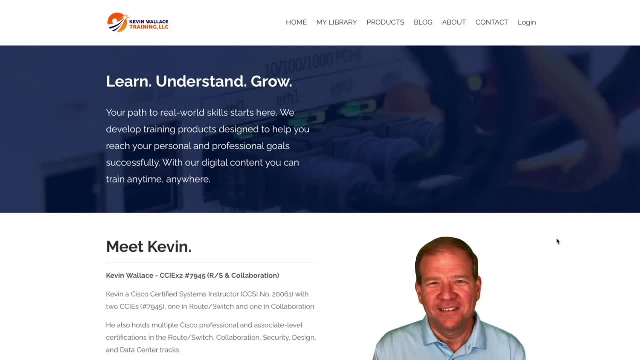 as its DNS server And its default gateway is 192.168.1.1.. And, like we did in a previous video, we want to do an ARP poisoning attack on traffic going between the victim's laptop and that gateway. Let's see what the victim's laptop IP address is. 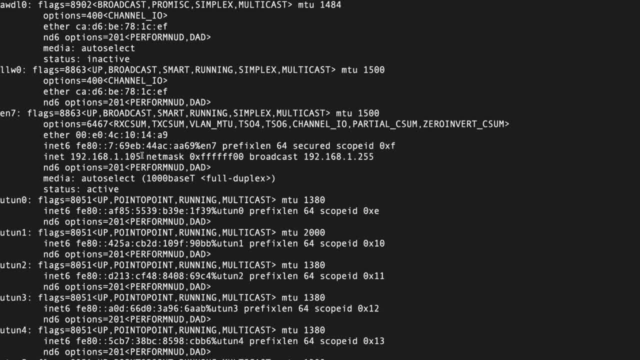 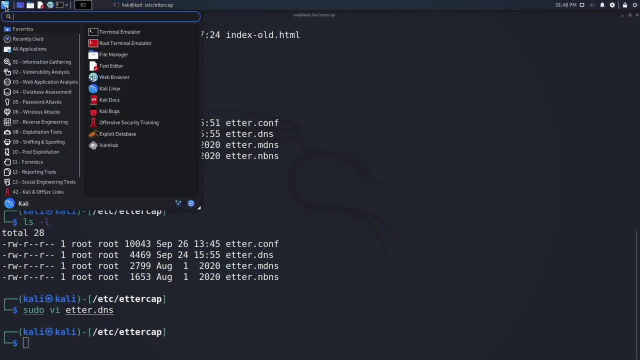 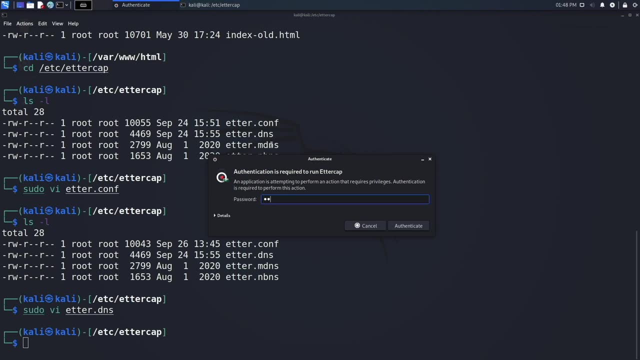 Let's do an ifconfig And it looks like it's 192.168.1.105.. So let's go back over to our Kali box And under the menu, under sniffing and spoofing, I'll say Ettercap, graphical- give the root password. 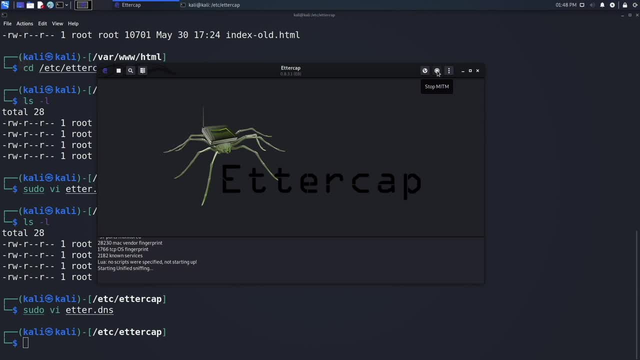 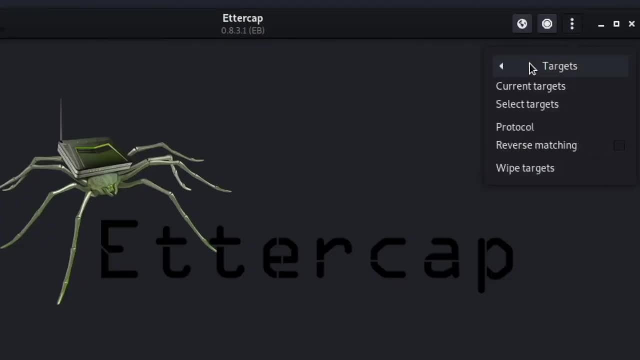 I'll accept that. Let's select our targets, And the targets are going to be the victim's laptop and the default gateway which is acting as the DNS server. So under this Ettercap menu, I'm going to say targets, select targets. And I'll say that the IP address of my victim's laptop is 192.168.1.105.. And my other target is the default gateway which is acting as that client's DNS server. It's at 192.168.1.1..